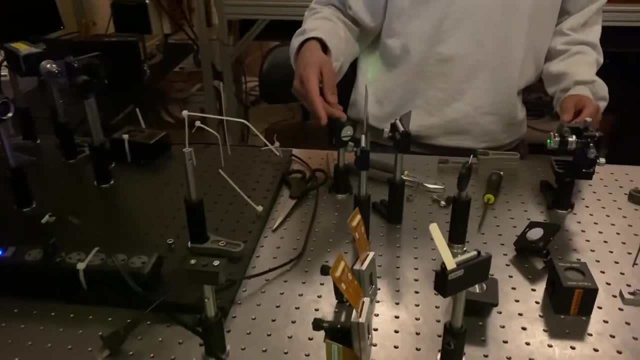 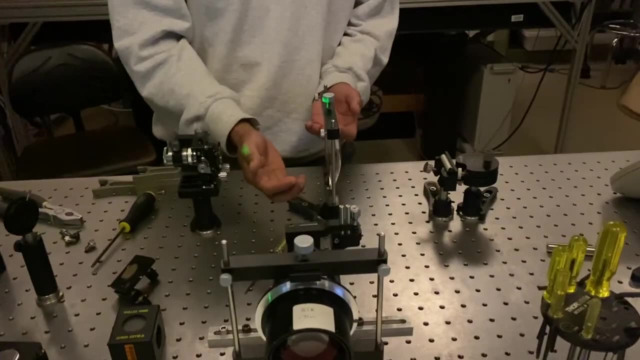 and then, after the beam splitter, we will come through and be reflected off a mirror into a microscope objective spatial filter and then we're going to be able to see the filter and then, after that, we will be collimating the beam through this collimating lens At 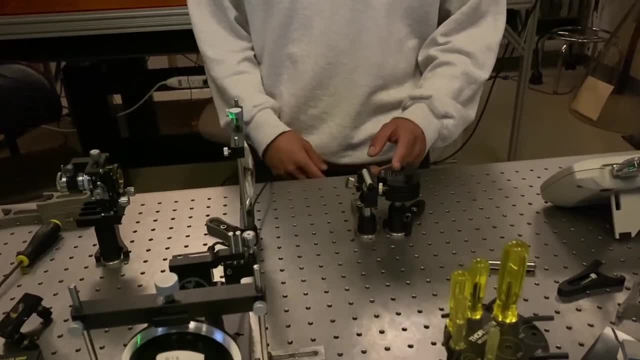 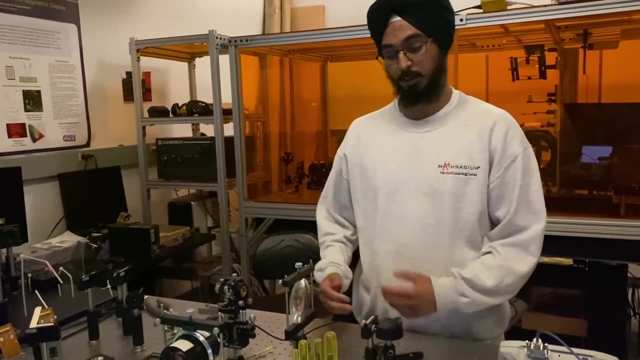 this point. here is where the photopolymer film lies, and our object will be placed here. So when recording a reflection hologram, there's two main components to consider, one being the power at the polymer film and the other the exposure time at the film. These two components- 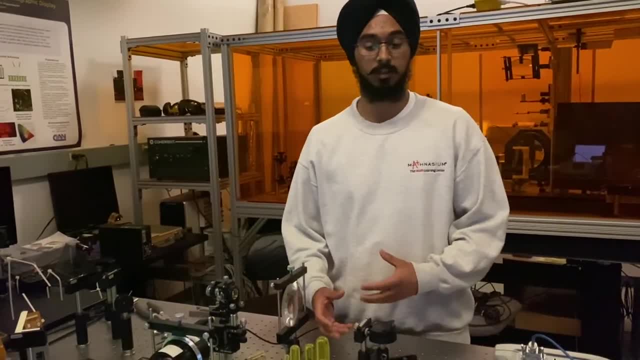 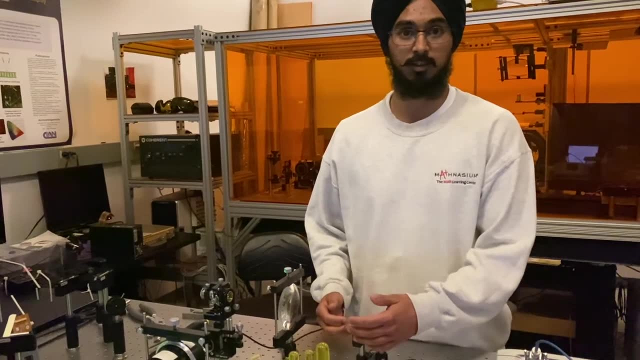 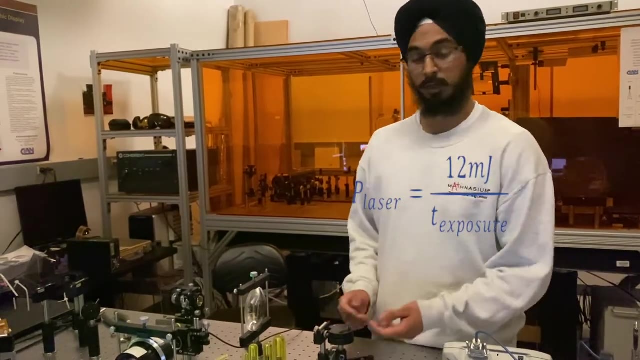 are related to each other by a property of the film, and that property is the energy required to induce a refractive index change on the film with the highest diffraction efficiency. So we had an energy level of 12 millijoules, and so during our experiment we did recordings. 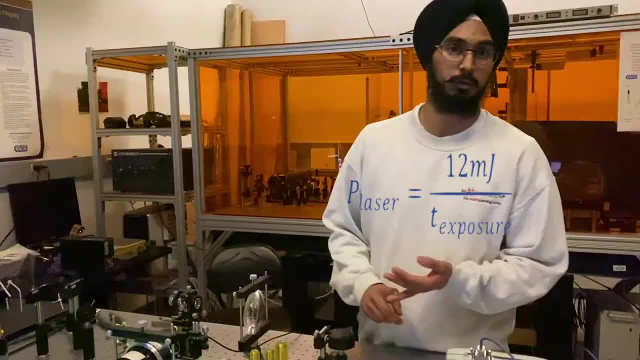 at a power of 0.6 milliwatts, 0.4 milliwatts and 0.3 milliwatts, and these correlated to exposure times of 20 seconds, 30 seconds and 40 seconds respectively For a recording. 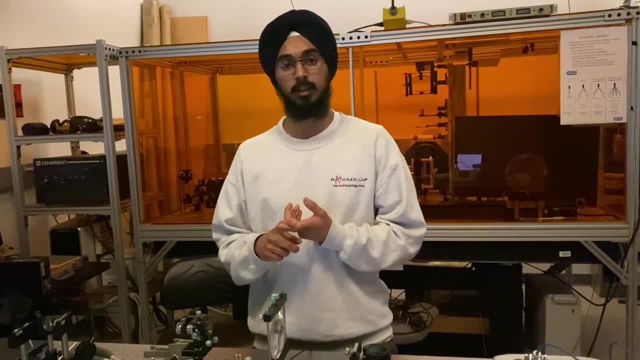 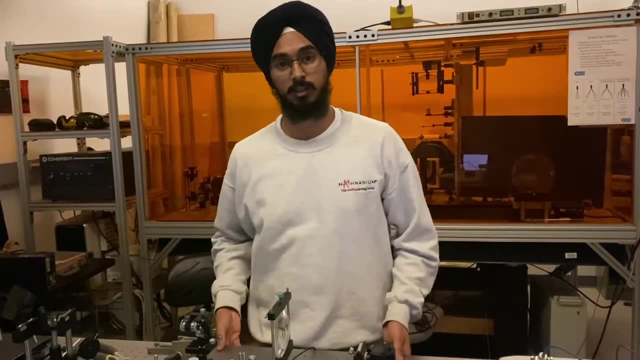 hologram. there should be very minimal external noise, so that includes lighting, sound and vibrations. So to reduce that, we would turn off all the lights in the lab and then we would allow this floating table to stabilize and also we would be dead-setting it. So that's. 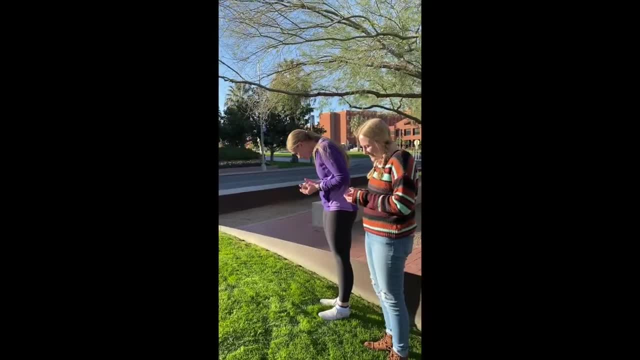 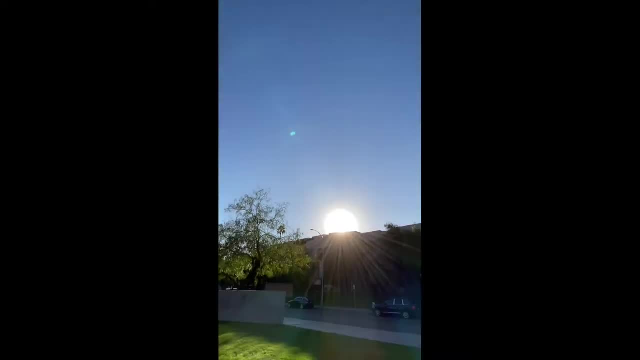 what we're going to do. In order to set the hologram, after the wanted interference has occurred, we exposed the film to UV light in order to bleach the film, so it cannot record any other images. So, after recording our holograms, we found that the sharpest hologram was created at 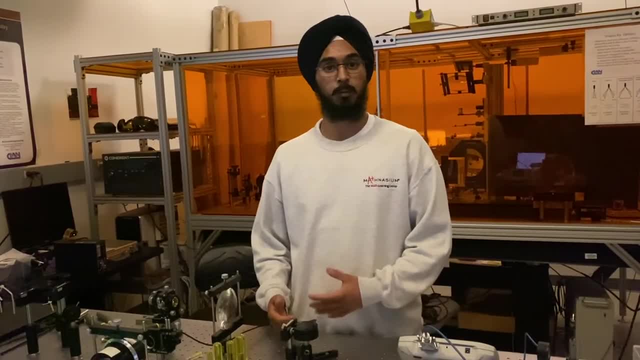 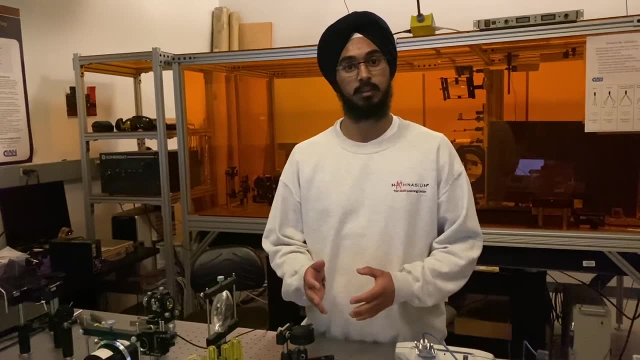 the highest power output and lowest exposure time. That was at the 0.6 milliwatt level and the 20 second exposure time. And as we increased exposure time while decreasing power, we found the sharpness kept decreasing. The reason that a hologram has dimension and depth is due to the fact that it has a 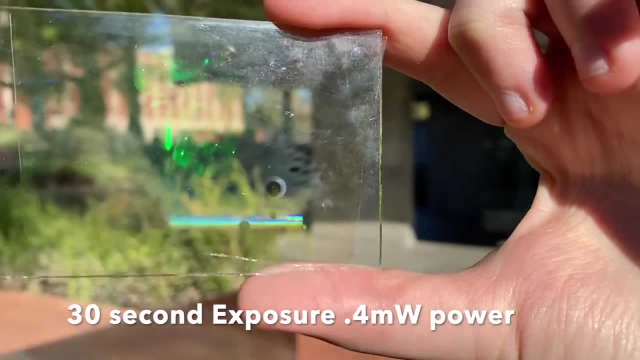 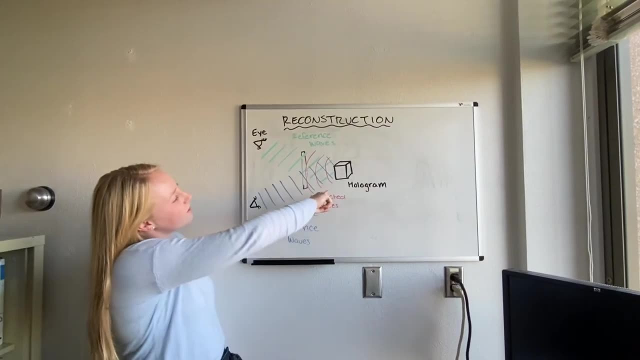 film that captures the wavefront of the object, whereas in a picture only the intensity is being recorded, causing it to be two-dimensional. For reconstruction of a holographic image, a reference wave must strike the holographic plate at the same angle as during the recording phase. This will reproduce the spherical waves. 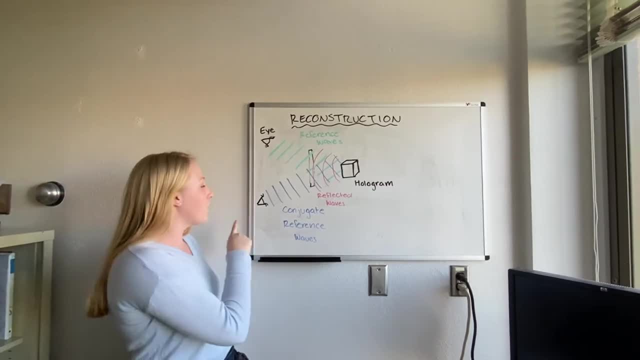 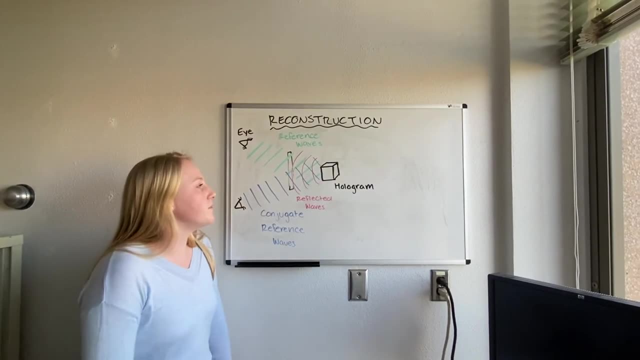 of the reflected object, which will be visible to the human eye. The conjugate reference wave will also produce a conjugate holographic image, though this image will be inverted. The holographic image can also be viewed on the opposite side of the holographic recording. 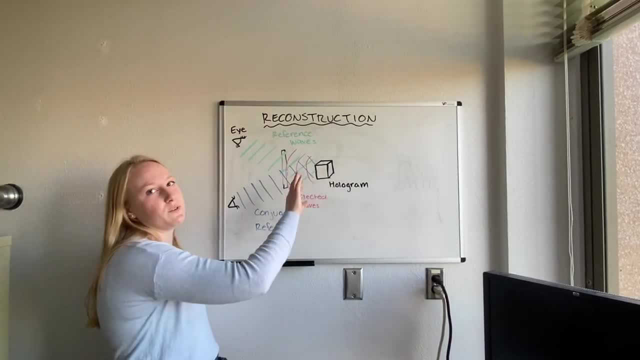 plate. due to the two conjunctions, The holographic image will also produce a conjugate image, though this image will be reversed in parity.